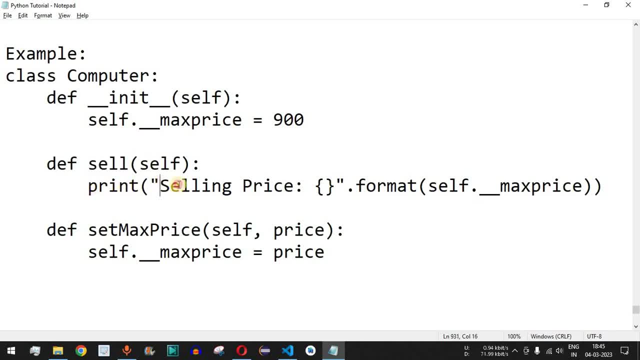 As you can see, we have the sell function over here, which simply prints the selling prices, the self, followed by dot and then the max price. So, basically, this statement will help us in order to print this value, that is, the max price value of the computer. And then we have another method, that is set max price, which takes the object that is using the self, and then it also takes the price over here. So, in case you want to set another max price for this computer, you can use this set max price function. What it will do is it? 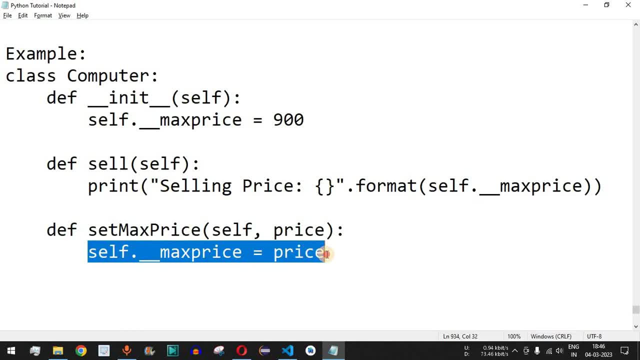 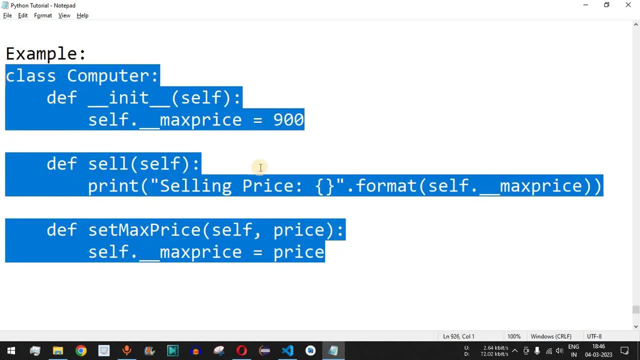 will simply update the value of the max price of the computer, as you can see, with this particular statement. so, guys, let us check this with the help of example. now what i will do is i'll simply copy these lines of code, since i am little bit lazy in order to type them again. so we are going to paste. 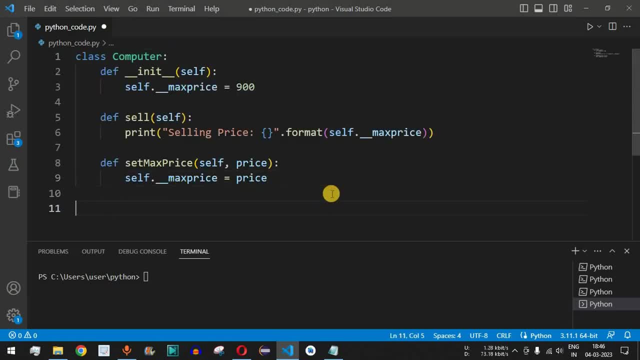 it inside the vs code. so over here, what we are going to do is we are going to print the max price of the computer. so first of all we are going to create the object, that is comp1 over here, followed by equal to, and then we have the computer class name. so basically, since the constructor is 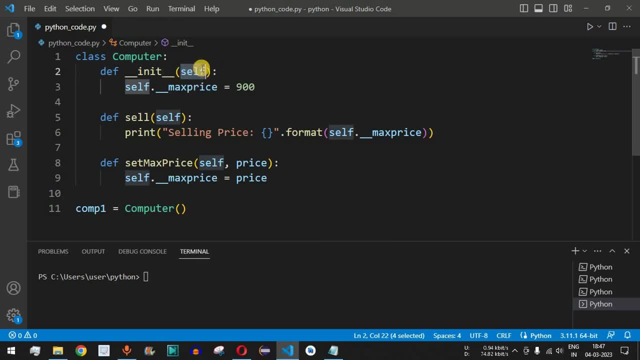 not taking any other parameter apart from this self, which is the object itself. so we need not have to provide any parameter over here while instantiating this object, that is comp1. now what we will do is simply we will call the cell function over here, that is, this particular function. so 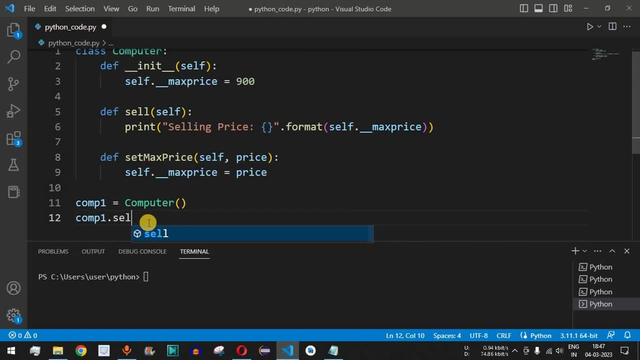 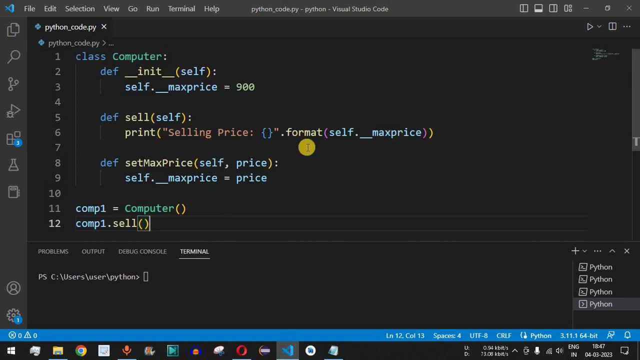 we can use the comp1 object followed by dot, and then we have the cell function. so after this, open and close parenthesis. so let me just save this file now and try running this code. so basically, this print statement should get executed and it should be displayed on the terminal. so i'll just run this code now. 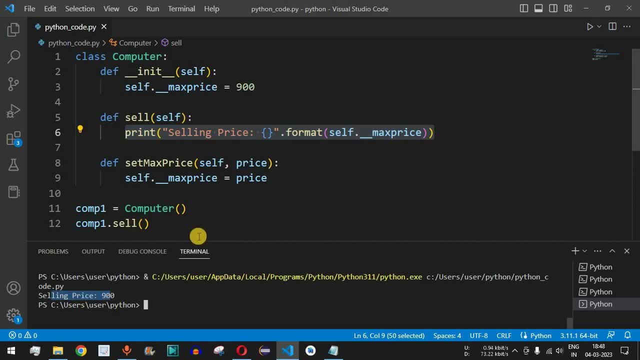 as you can see, selling price is 900. so what exactly happened is, when the control flow came over here, that is comp1, it is equal to computer- the constructor of this class, that is the init method, was called, and inside this, what we have done is this private attribute. so, guys, basically, 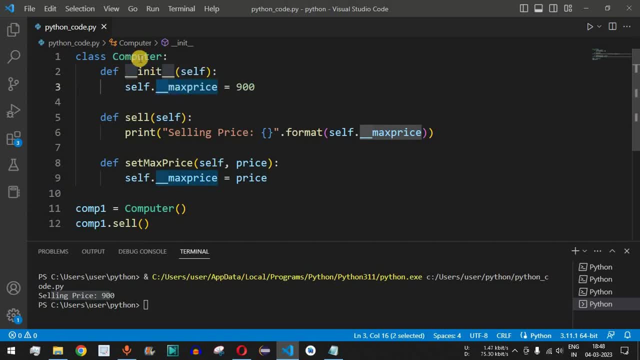 this double underscore denotes that this is the private attribute of the computer class. so basically this private attribute was initialized inside the constructor and the value of 900 was being assigned to this particular attribute. and then what we did is, when the control flow came over here, that is, while calling the cell function, basically this print statement was executed. so 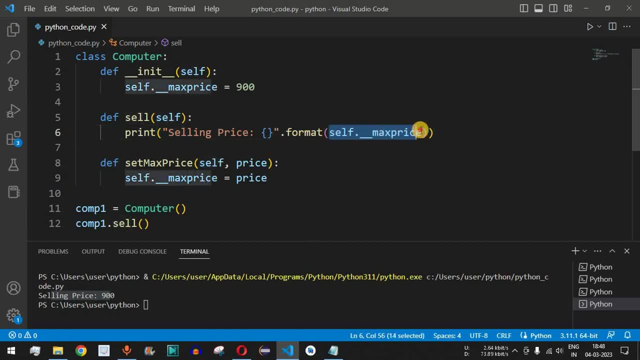 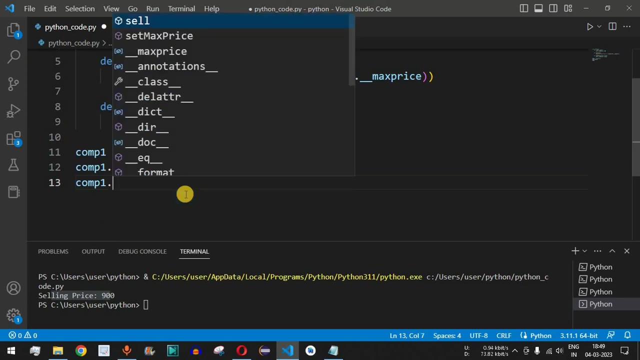 selling price. it is equal to this self dot max price got printed over here, which is 900 right now. now, guys, let us do another thing. what we will do is we will try to access this private attribute from outside of this class. so over here we will call comp1 once again, followed by dot, and then we can. 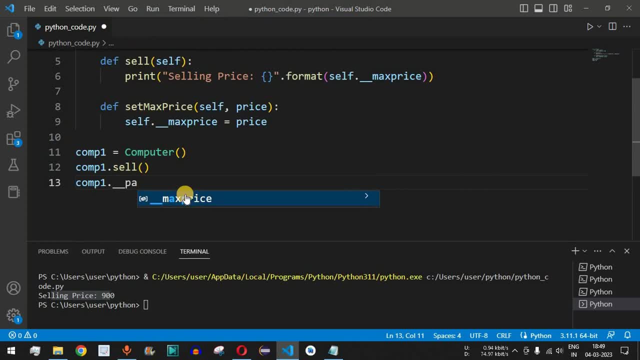 call this private attribute, that is the max price. so, as you can see, this max price is getting suggested by the vs code. so we will call this max price and what we will do is we will try to assign another value, that is 1000 over here, to this max price. and then again, let us say we want to call this print. 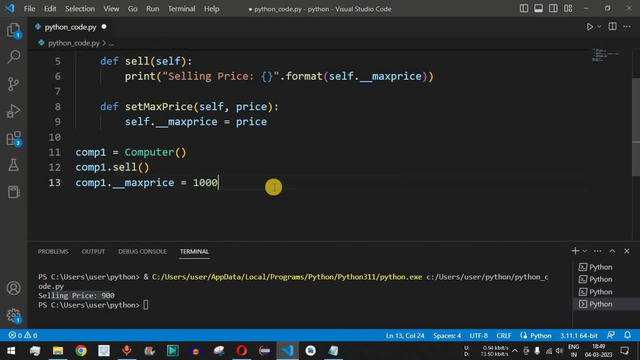 statement. so again, we will call this cell method over here. so i'll just copy this line of code and me just save this file now and try running this code. so, as you can see, selling price: 900. this is a statement that was printed by calling the first cell method and then the second time the cell. 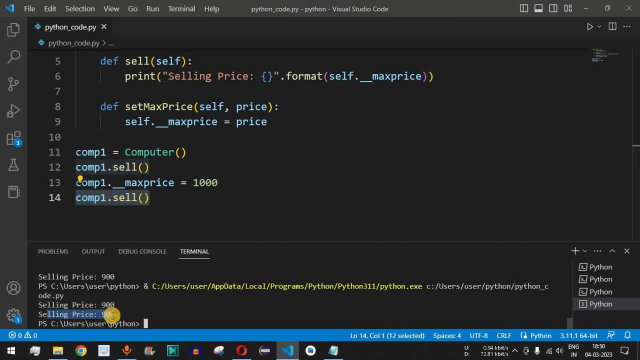 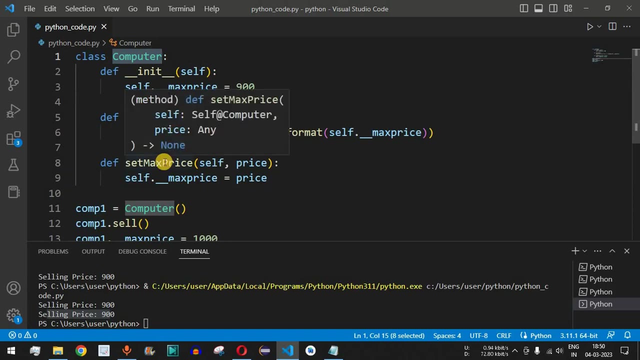 method was called again, the selling price was equal to 900. so, guys, why so? that's because this max price is the private attribute and we directly cannot access this attribute by using this object. we need to have another method inside the computer class in order to assign another. 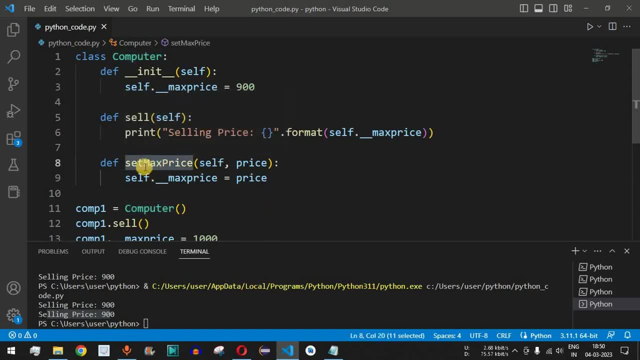 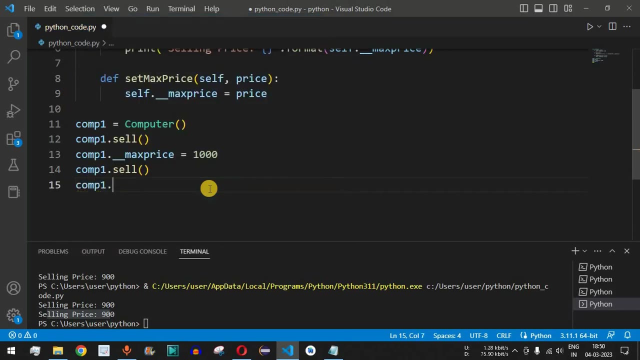 value to the private attribute, and that is why we have this method, that is, the set max price along with the parameter price which it is going to take in order to replace the existing max price over here. so what we can do is we are going to call the comp1 object once again, followed by dot. 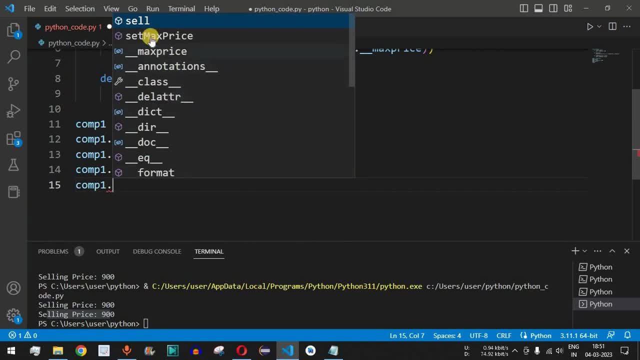 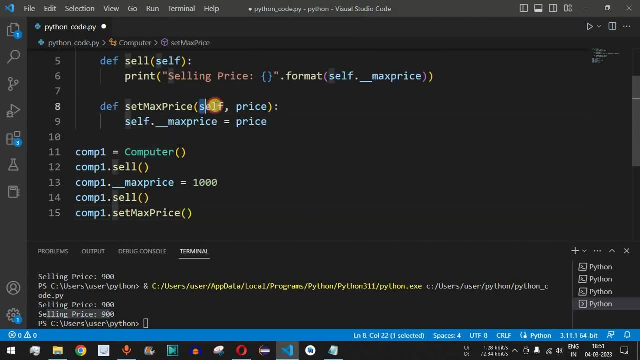 and this time, instead of directly accessing this max price, we are going to call this set max price over here. so set max price, and it is expecting two parameters. the first parameter is the self, which i'm going to call the private parameter, and then set price, also followed by dot. 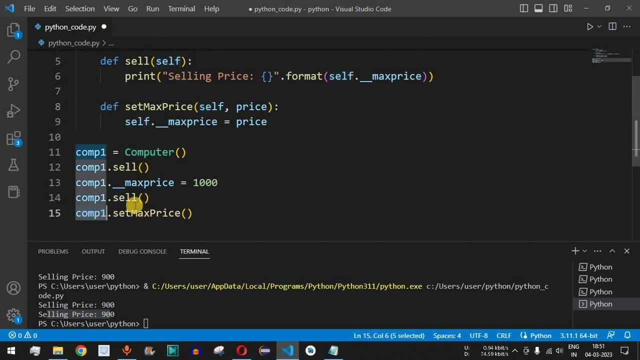 is going to be passed by default, which is going to be the comp one object, and then the second parameter is the price, which we are going to pass to this method. so, again, what we will do is, simply, we are going to provide this thousand price that we try to assign to the max price directly over. 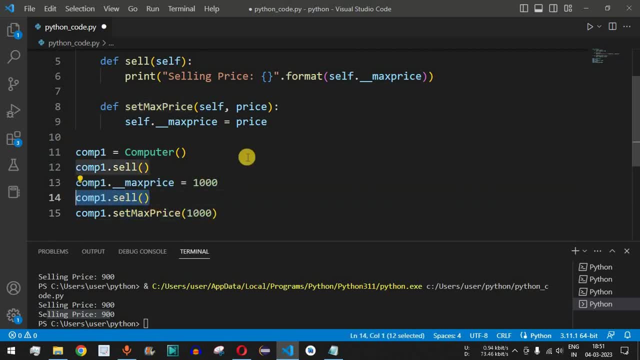 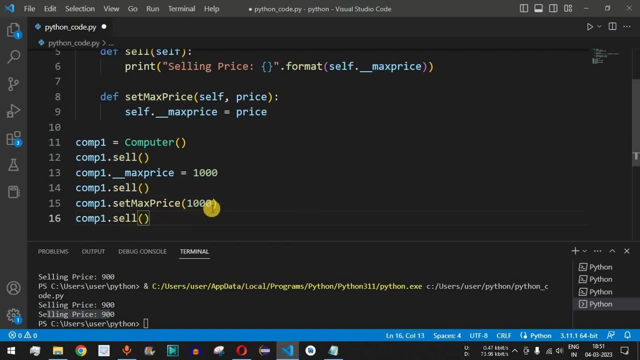 here, so set max price. and then again let's say we want to print the selling price over here, so again we are going to call the sell method once again. so comp one dot, sell, so over here. the only difference is we are calling the method, that is, the set max price, and we are passing the value of the new max. 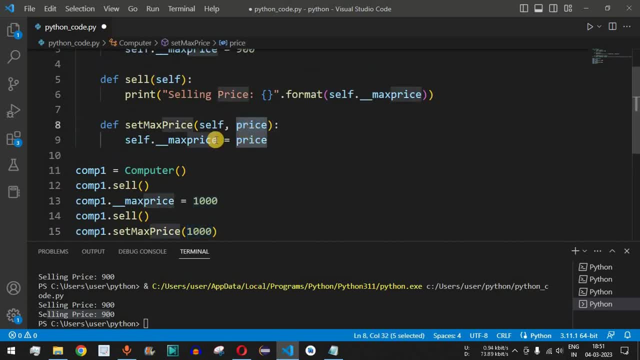 price over here which is going to be passed to this price, and then the max price value will be the updated price that we have just set. so, guys, let me just save this file now and try running this code, so as you can see: selling price 900, and then selling price 900 once again. and the third: 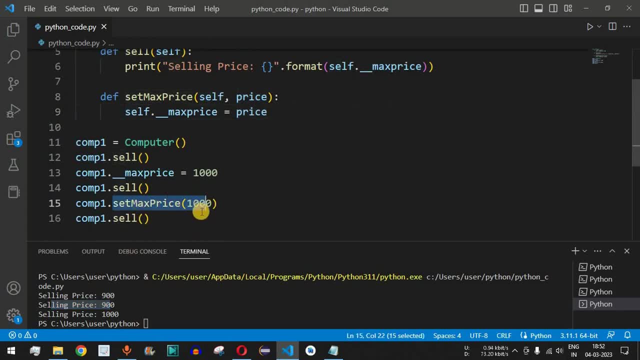 time that we tried by using the set max price over here it was 1000, so this time it is selling price. it is equal to 1000. so, guys, by using the set max price over here, we are going to be able to set the selling price over here and then. 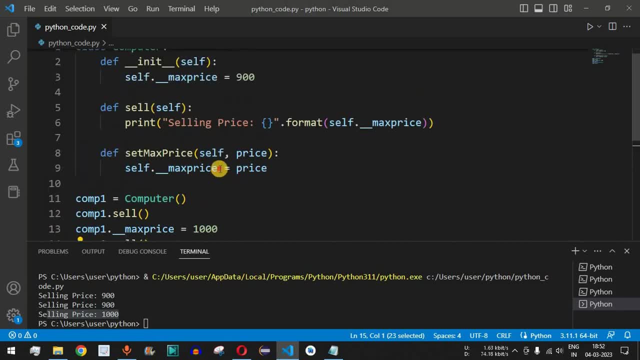 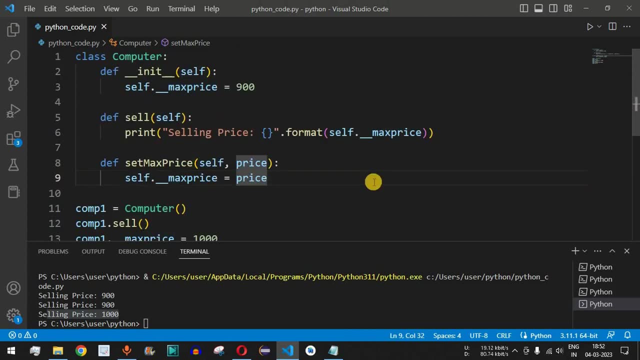 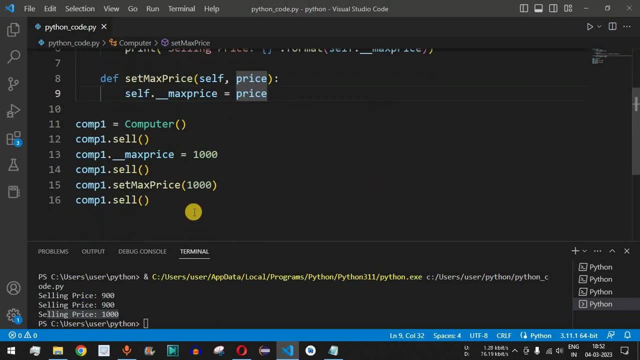 this method in order to set the value of a private attribute. we were successfully able to update the value of this private attribute, and this is the main functionality, which we call it as encapsulation, as far as object oriented programming in python is concerned. so, guys, let us run this code once. 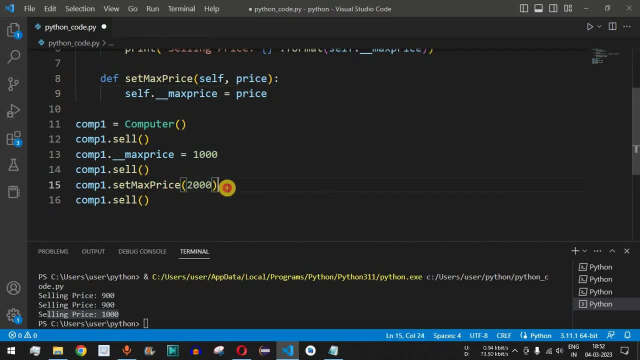 again by a different value, let's say the max price. over here we set it to 2000, so let me just save this file now and try running this code. so this time the selling price is coming over here once again as 2000. and guys, this is the way in. 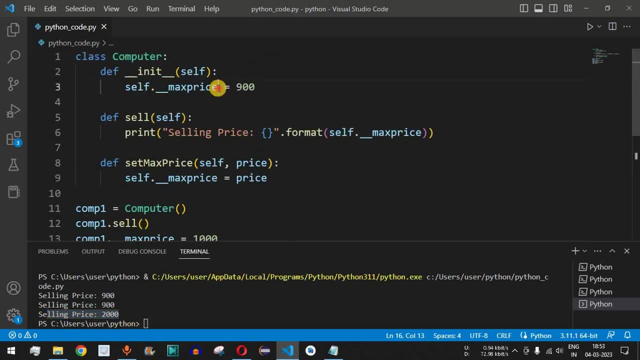 order to hide certain attributes of a class, you can have them as the private attribute by prefixing, and use the different methods in order to set their values by using the objects of that class. so, guys, practice on your own so that on different inputs you get different outputs. please make sure. 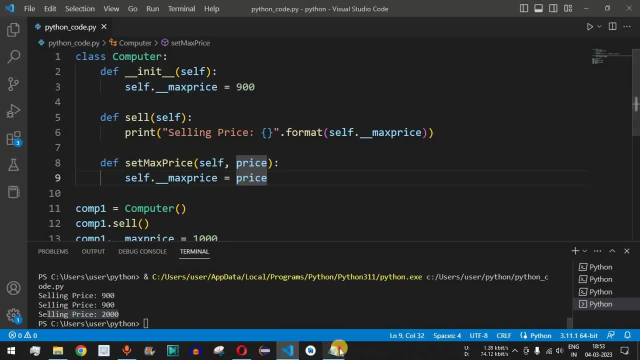 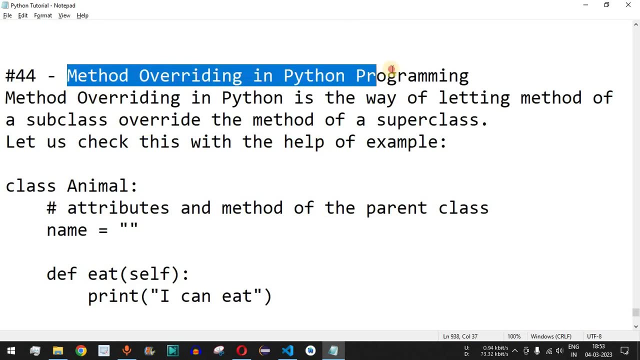 that you like this video so that it reaches to more people, and subscribe to this channel so that you get the notifications on upcoming videos as well. the next video that we are going to talk about is method overriding in python programming, so stay tuned you.